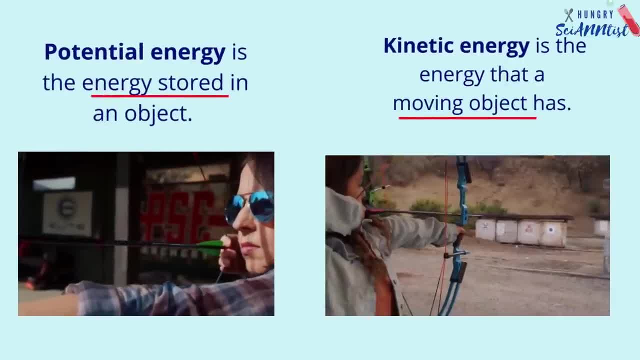 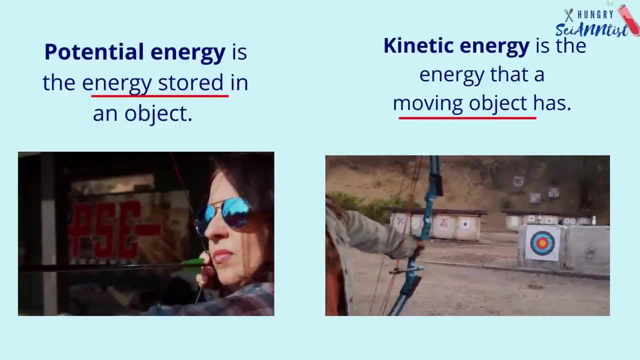 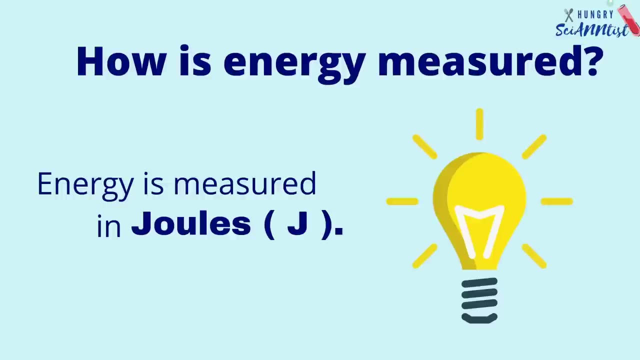 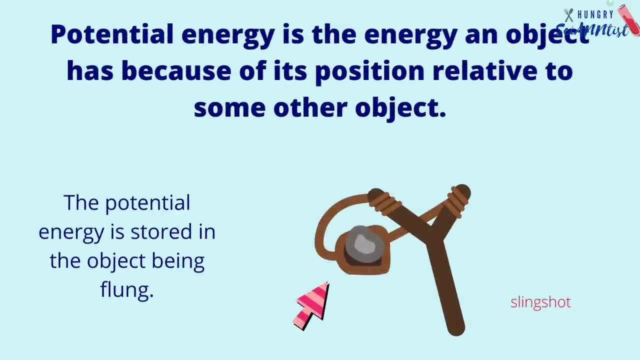 Potential energy is the energy stored in an object. Kinetic energy is the energy that a moving object has. How is energy measured? Energy is measured in joules. Potential energy is the energy an object has because of its position relative to its position. 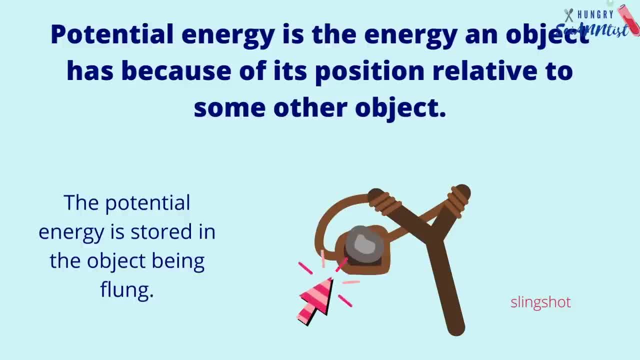 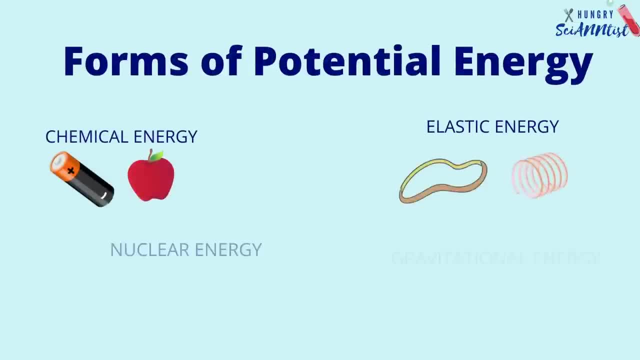 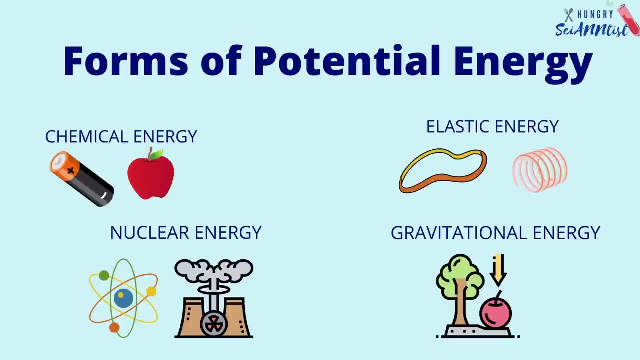 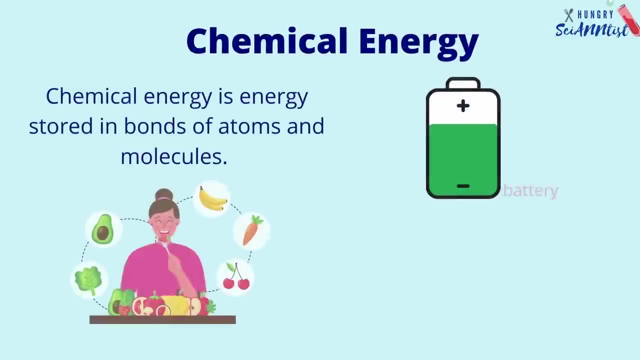 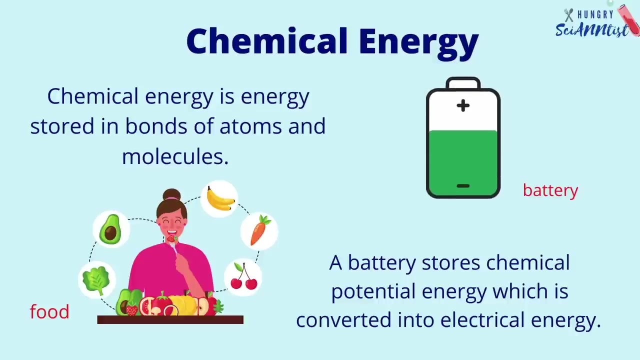 In a slingshot. the potential energy is stored in the object being flung. Forms of potential energy: Chemical energy, elastic energy, nuclear energy and gravitational energy. Chemical energy- Chemical energy is energy stored in bonds of atoms and molecules. A battery is also displayed in a slingshot. 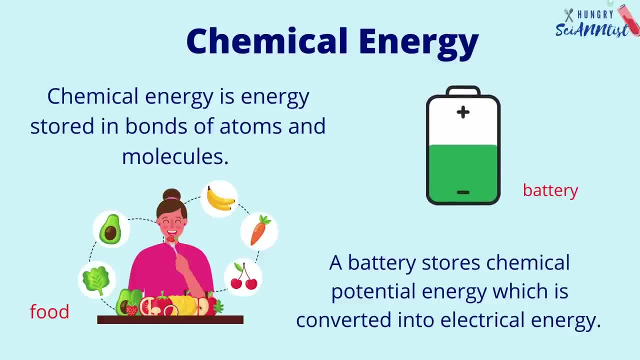 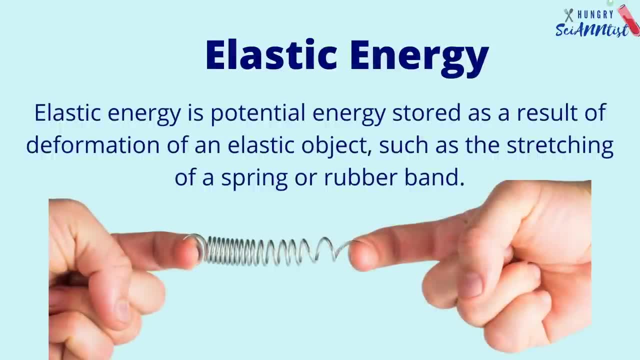 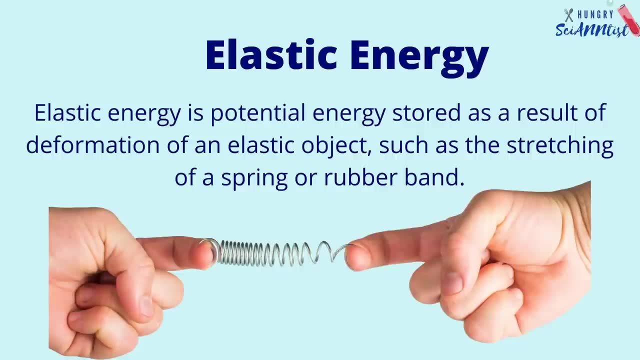 A battery stores chemical potential energy which is converted into electrical energy. Potential energy is stored in both slaves: Elastic energy. A battery has 3 positions on each slingshot. Potential energy is stored as a result of deformation of an elastic object, such as the stretching of a spring or rubber band. 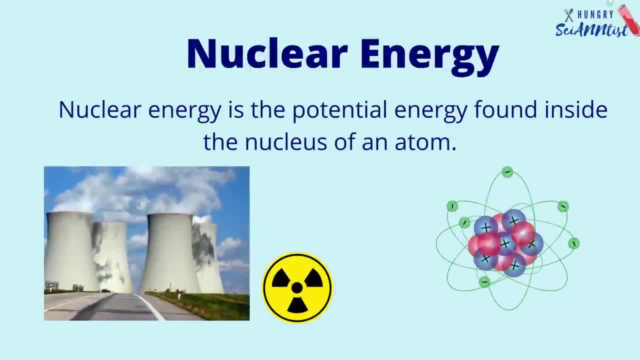 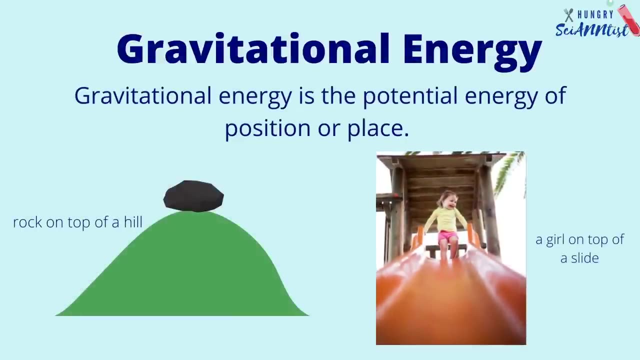 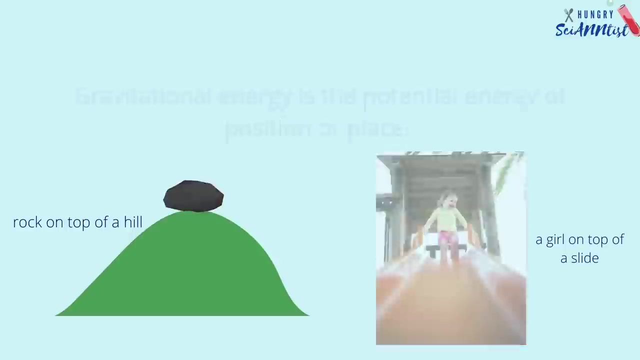 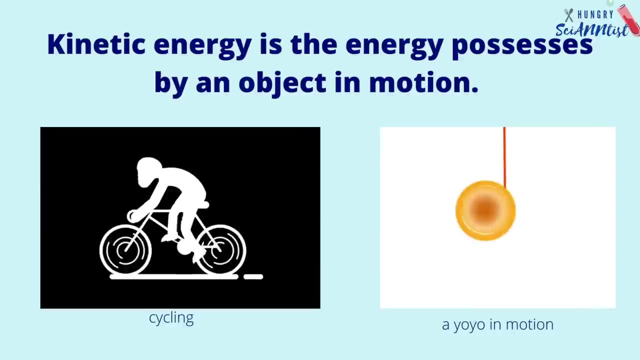 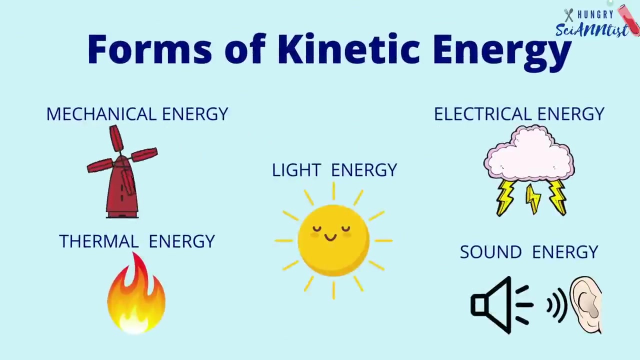 Nuclear energy. Nuclear energy, the potential energy found inside the nucleus of an atom. gravitational energy is the potential energy of position or place, like a rock on top of a hill and girl on top of a slide. kinetic energy is the energy possesses by an object in motion. forms of kinetic energy, mechanical energy, thermal energy, light. 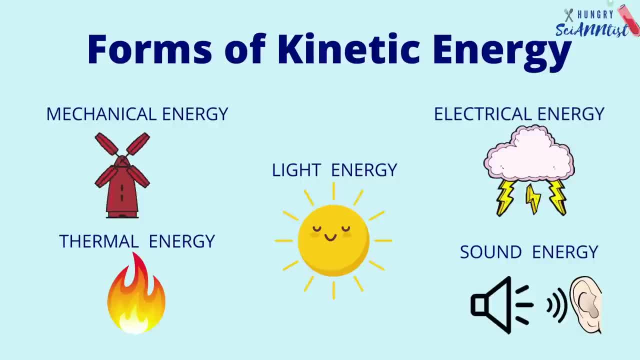 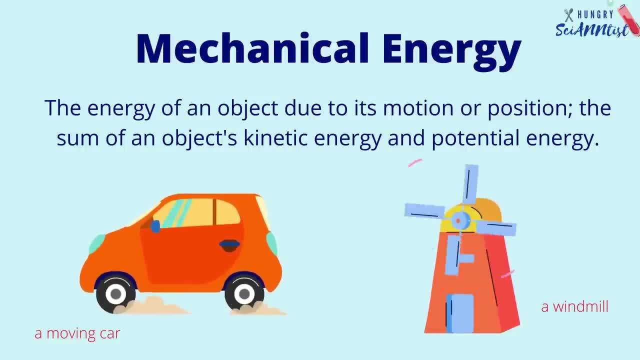 energy: electrical energy and sound energy. mechanical energy is the energy of an object due to its motion or position. the sum of an object's weight is not pushed from the ball to the rel. Finalżyk is an individual energy carrying an energy from an aggregate to the largest single object in the galaxy.